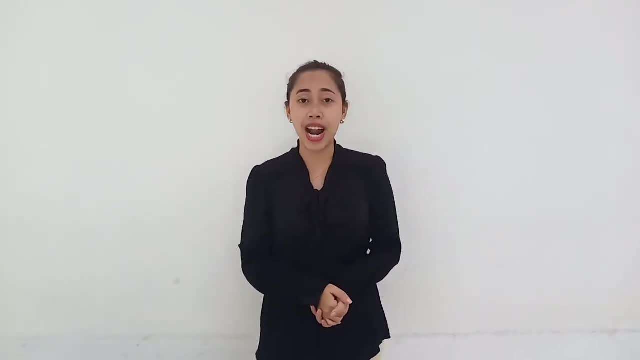 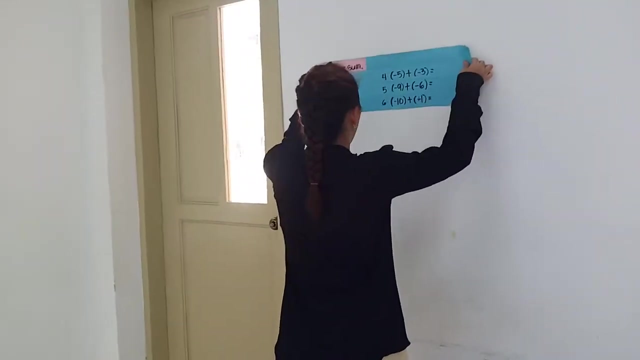 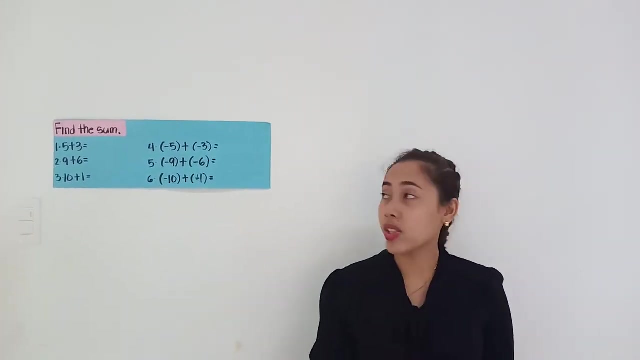 The answer is 38.. Okay, I must say that your addition skills are all improving, So in relation to that, you will have an activity. Please answer this for 3 minutes in a scratch paper. So time is up. What is the answer for number 1?? 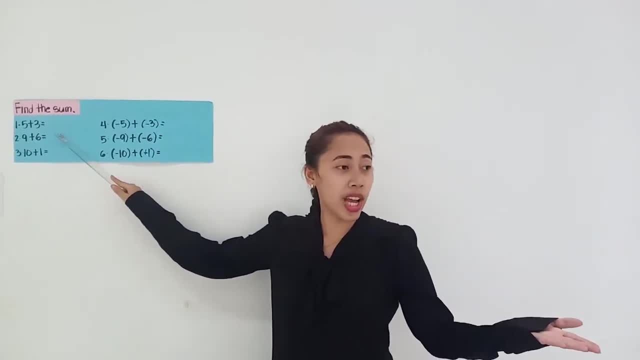 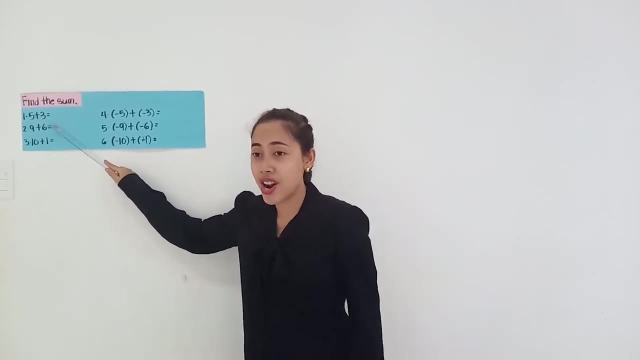 5 plus 3 is equal to. Yes, Janus, Okay, very good. 8.. How about 9 plus 6?? Okay, Janessa, What's the answer? Okay, 15.. How about 10 plus 1?? 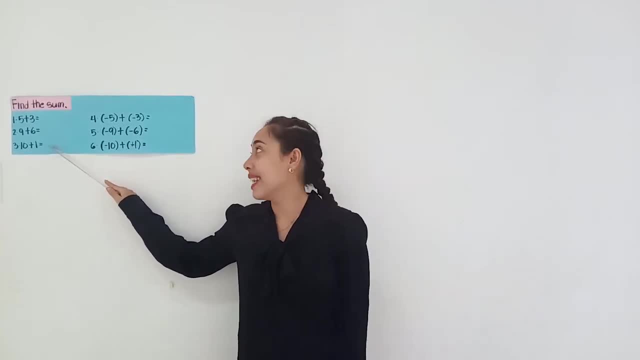 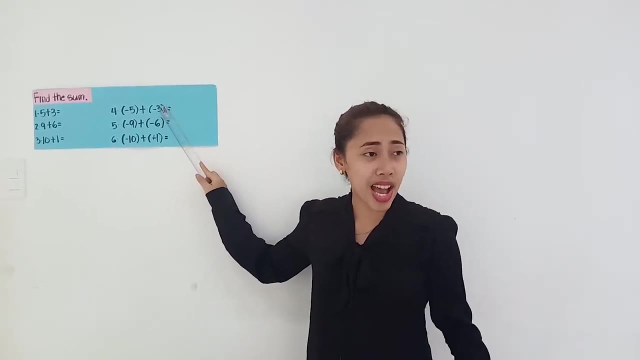 Remark. Very good, The answer is 11.. How about number 4? Negative 5 plus negative 3.. Aliza, What's the answer? 8?? Who has another answer? Thank you for that, Aliza. Who has another answer? 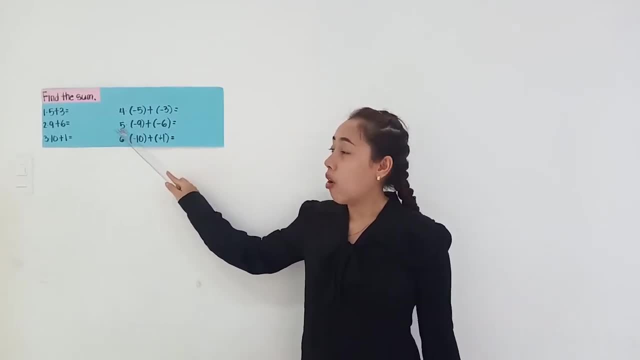 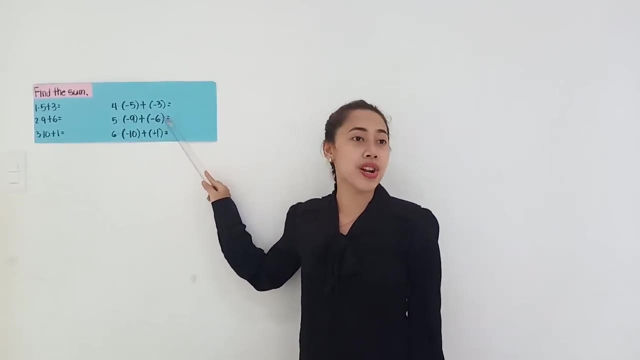 No one. Okay, let's skip it for a while. How about number 5?? Negative 9 plus negative 6.. Who has an answer? Again, no one. Janus, What's the answer for number 5?? Okay, you don't know the answer, so please be seated again. 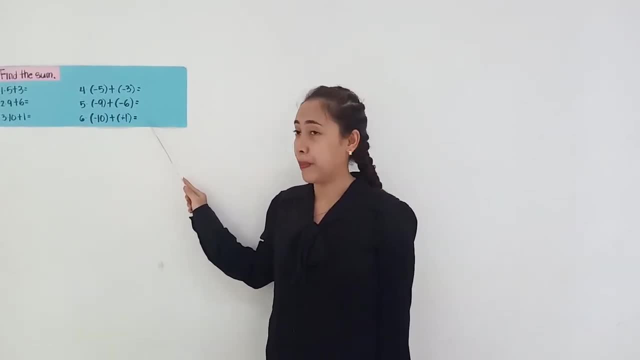 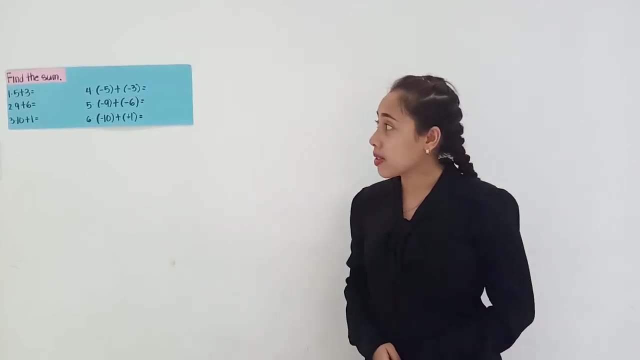 So 4,, 5, and 6 is just the same. So we will know the answer after we dig deeper into our topic for today. So, based on our activity, what do you think is our topic for today? Yes, Abigail. 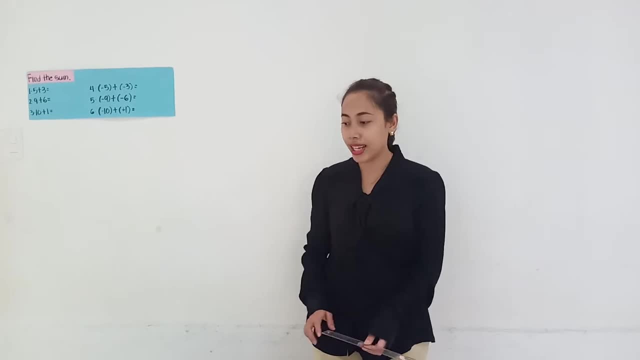 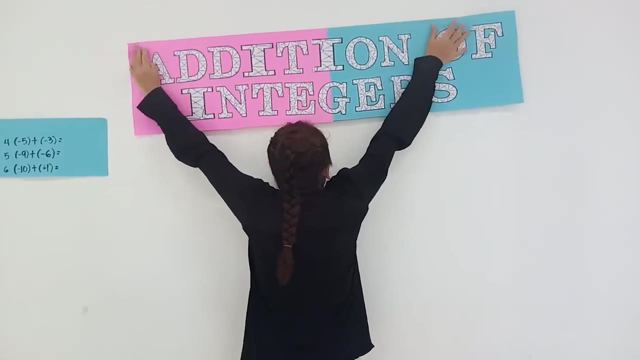 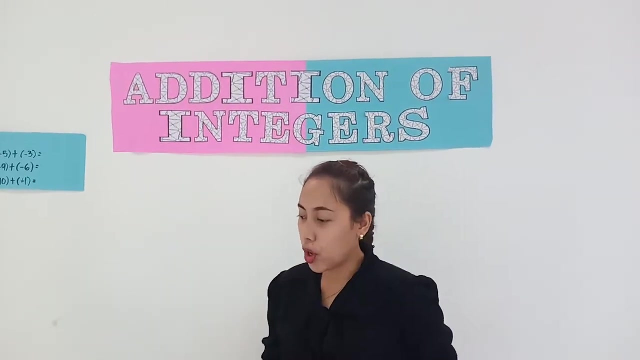 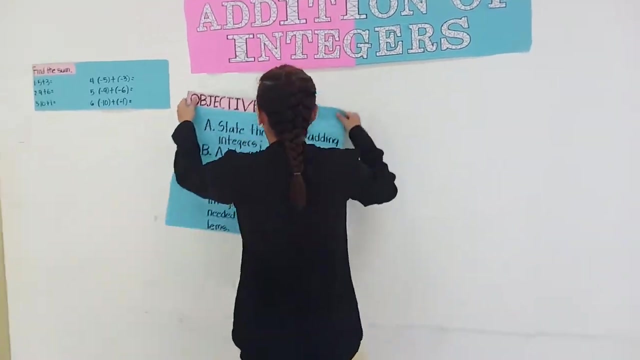 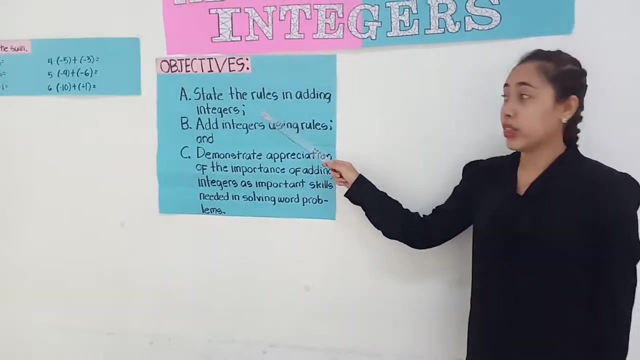 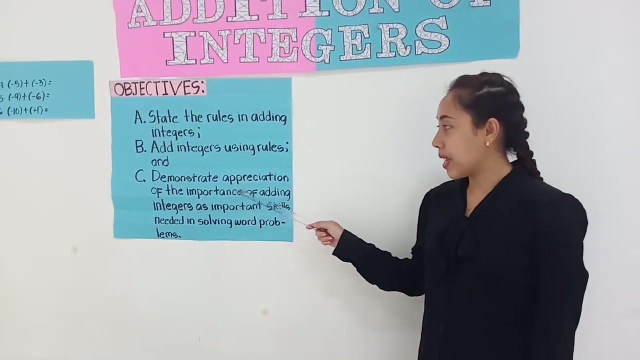 Okay, very good, Our topic for today is all about addition of integers, So before that, we will now receive the objectives for today. So the first objective is state the rules in adding integers, Then add integers using rules And last, demonstrate appreciation of the importance of adding integers as important. 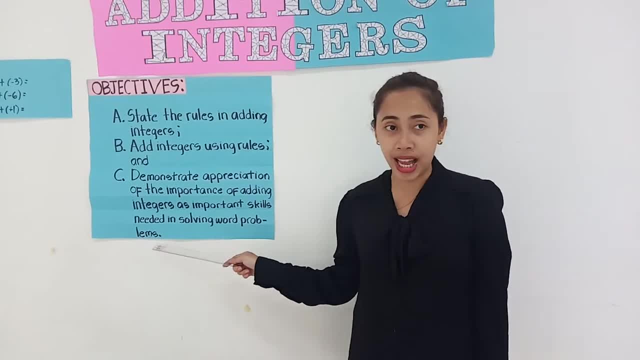 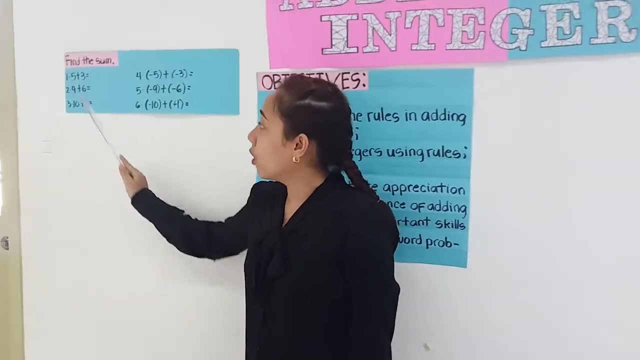 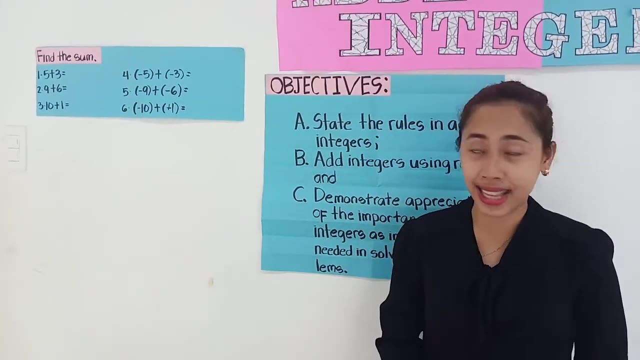 Now we will go back to our activity a while ago, which is this one. So you only got 1,, 2, and 3 correct. How about number 4,, 5, and 6?? So I will give you a hint. So the answer for number 4 is negative 8.. 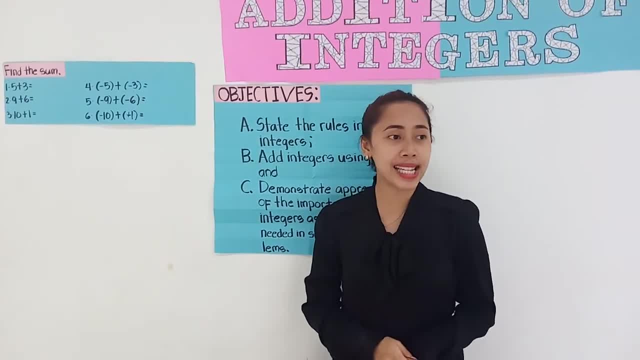 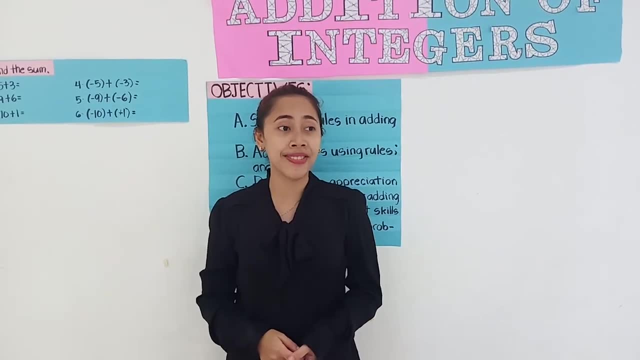 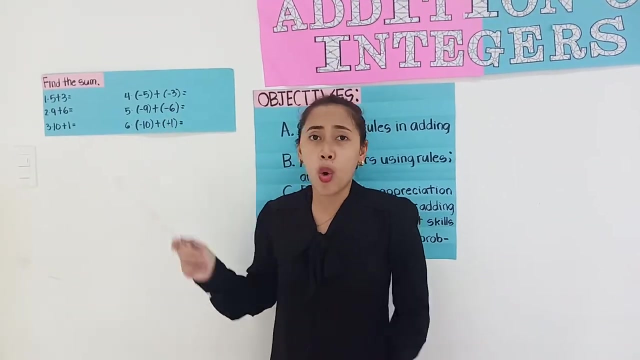 Why do you think the answer is negative? 8?. Who has an idea? Yes, Eliza. Okay, very good. You just added their absolute value and you copied the signs, since they are the same. So, in relation to that, what do you think is the first rule in adding integers? Yes, Raymar, What's the answer? Okay, very good, You have a point. So the first rule in adding integers is adding their absolute value. Then you copy the common sign. When we say common, it means they have the same sign. 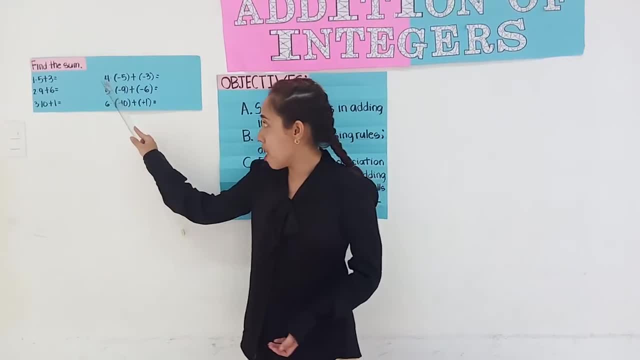 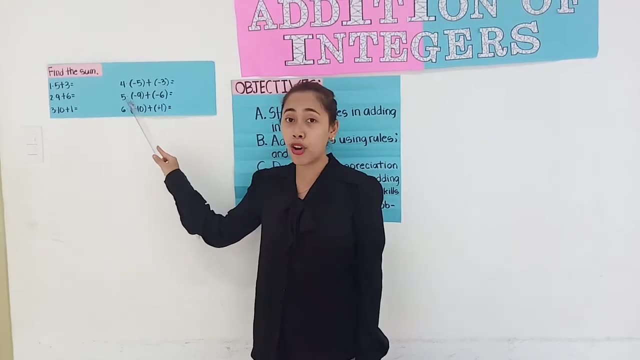 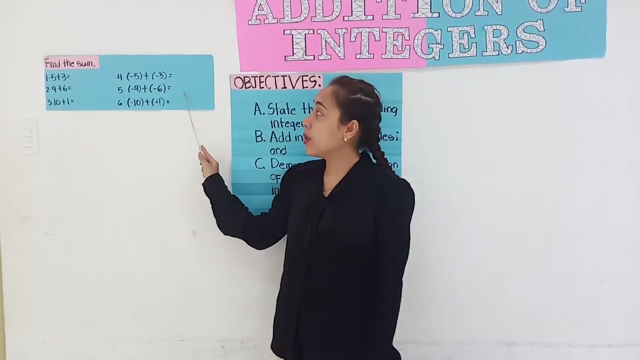 So you already know the answer for number 4.. How about number 5?? Negative 9 plus negative 6.. So it is the application of our rule, number 1.. Yes, Raymar, What's the answer? Very good, So now the answer is negative, 15.. 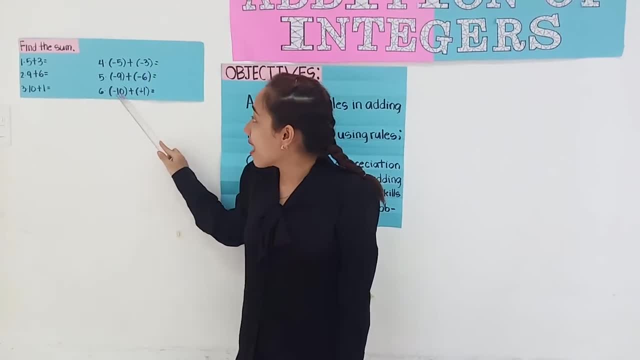 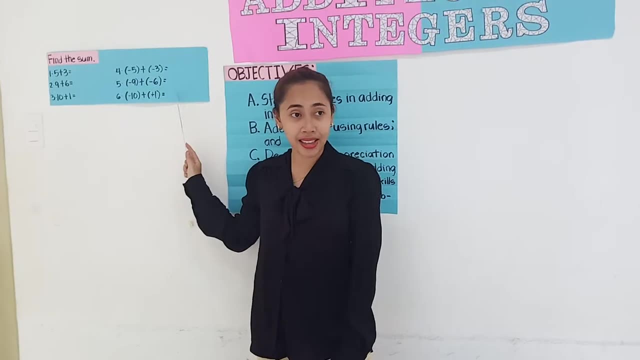 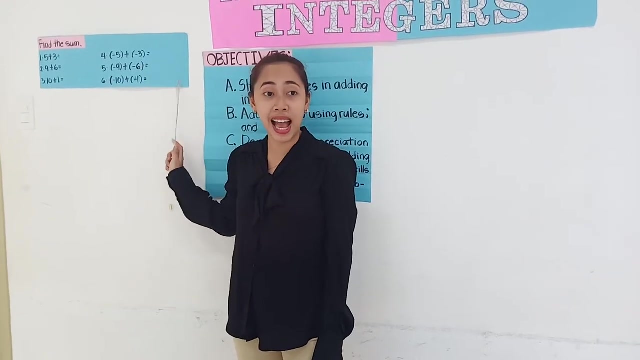 How about number 6?? Negative 10 plus positive 1.. Oh no, they are now having unlike signs. So what do you think is our answer for this? What are we going to do with this? They are having the same sign. 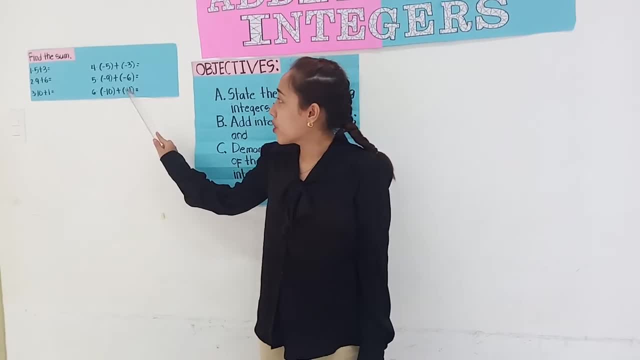 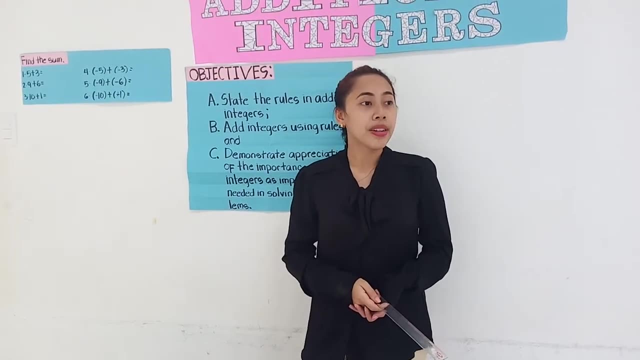 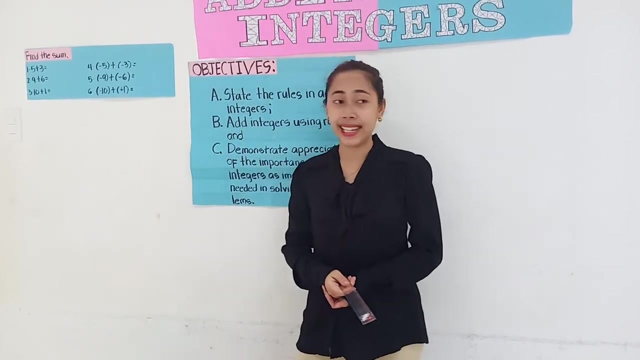 Okay, Janessa, What's the answer? So the answer for this one is negative 9.. So how did you get negative 9?? Okay, very good, You added their absolute value. Then what? How did you arrive with negative sign, Janessa? 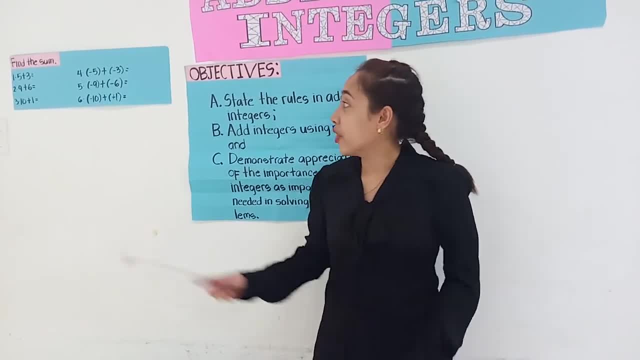 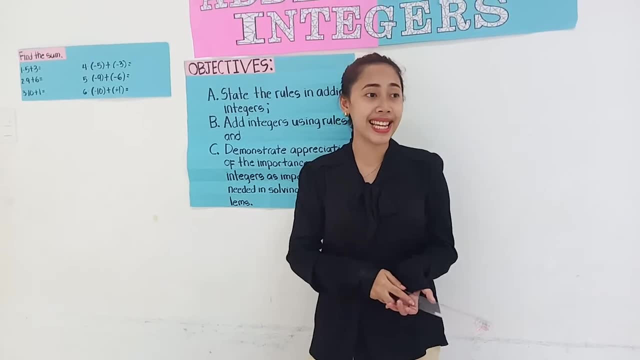 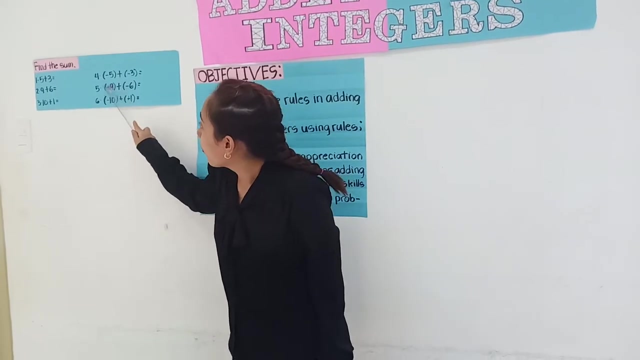 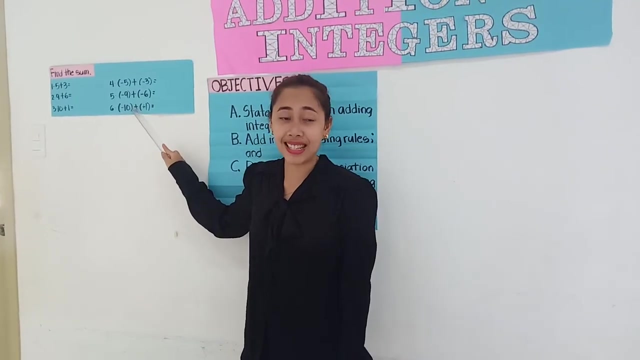 Oh, you copy the sign of the greater number, which is 10.. So, very good, That is our second rule. in adding integers Having unlike signs, You just have to add, You just have to subtract their absolute value and copy the sign of the greater number. 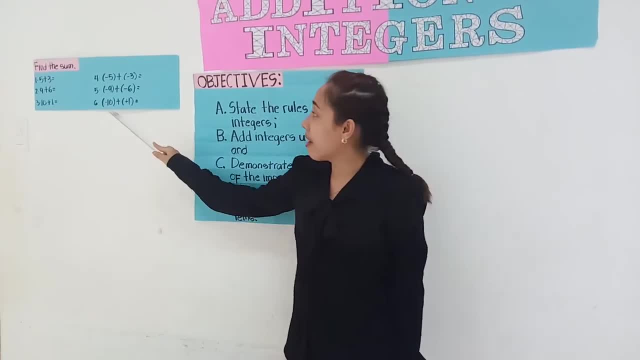 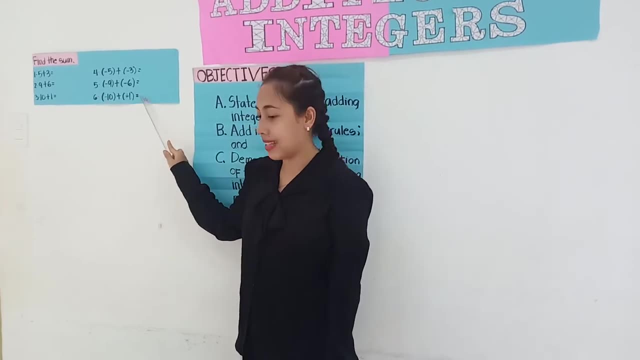 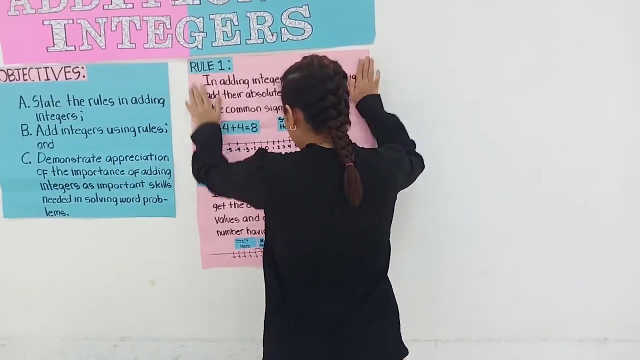 So this one, 10 minus 1, is equal to 9.. They are having unlike signs which is greater, 10 or 1.. So 10.. So we will just copy the negative sign. So please read The rules in adding integers. 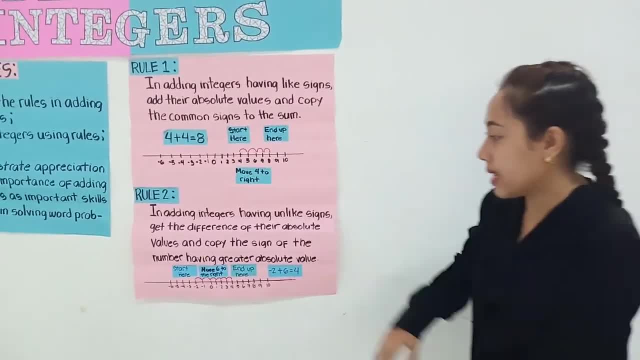 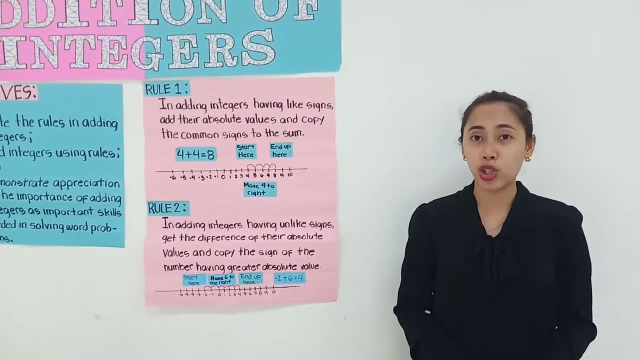 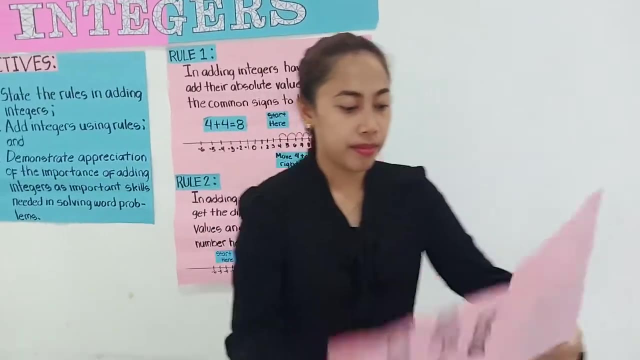 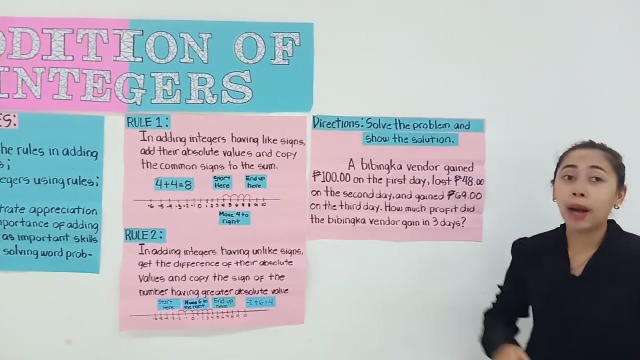 So these are all the rules in adding integers. So please take note of this rule, because we will be using this one in adding integers in relation with problem solving. So now, So apply the rules in adding integers to this problem and solve it for 5 minutes. 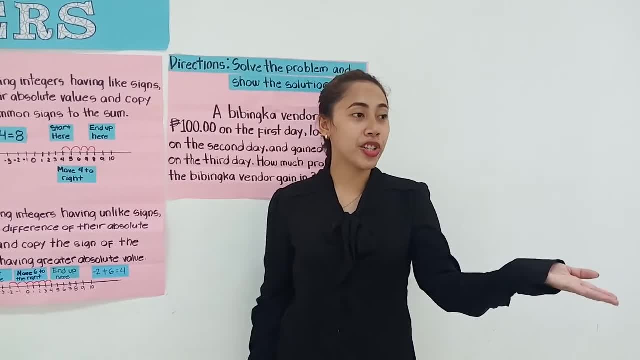 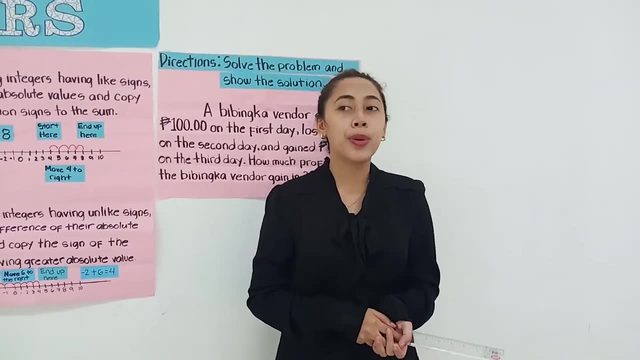 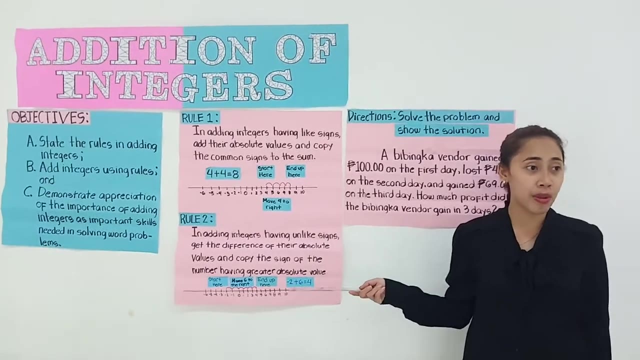 Okay, time is up. What's your answer? Janessa- Okay, very good. That's the correct answer. Do you have the same answer with Janessa- Okay, very good. Any questions about the packet addition of integers or any clarifications before we proceed? 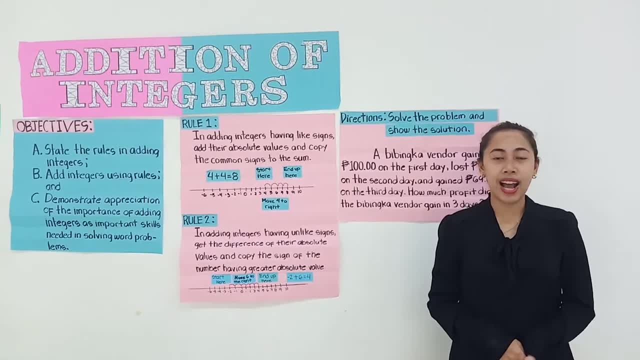 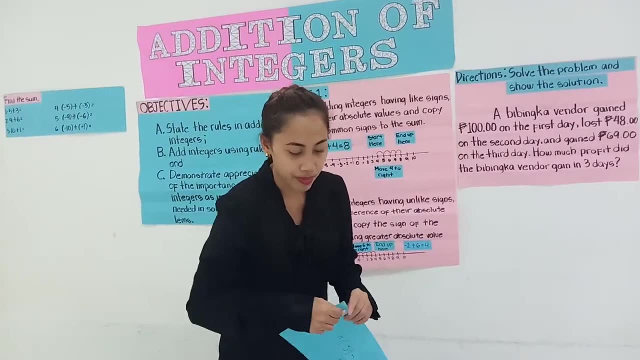 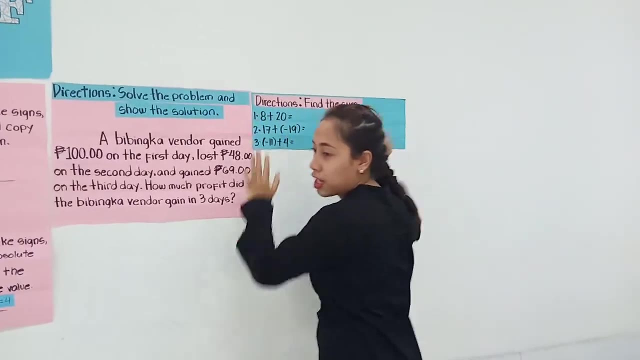 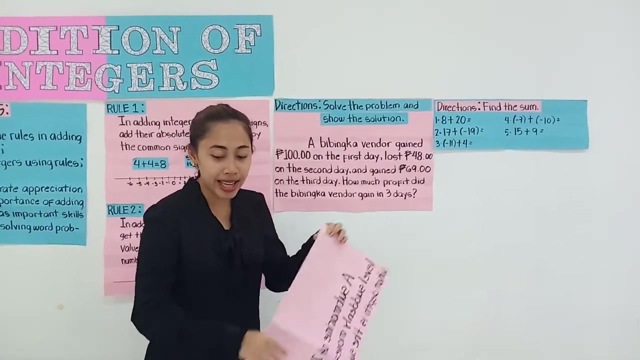 Okay, done So. now please get one half sheet of paper and answer this one for 5 minutes. So this is the first part And also answer the second part for 5 minutes. So you have a total of 10 minutes in answering this one. 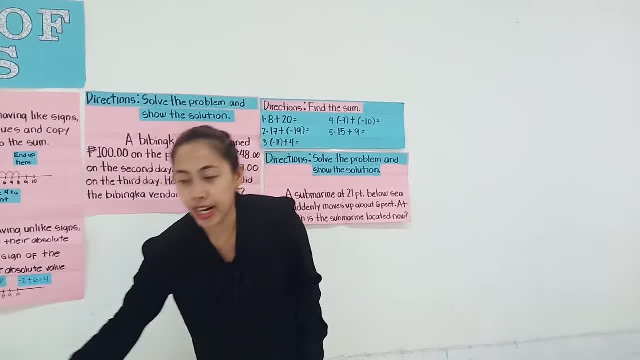 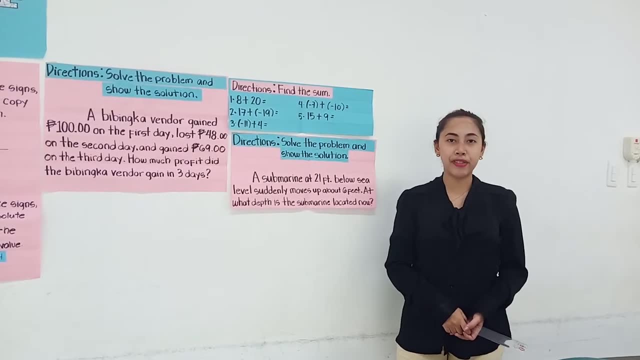 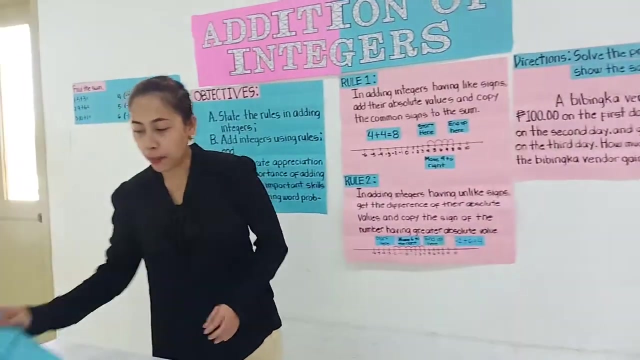 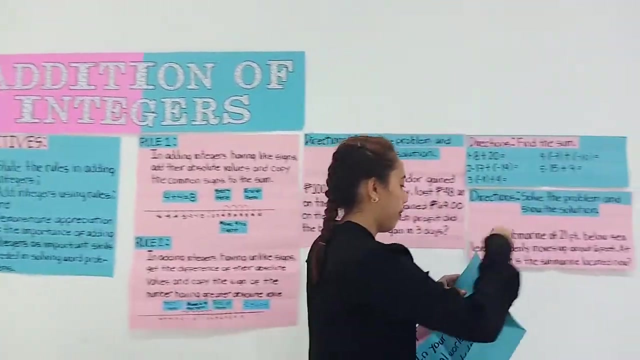 So please use one whole sheet of paper in answering. Okay, time is up. What's your paper? syndrome 1,, 2, 3.. Okay, all papers are submitted. So please copy your assignment for tomorrow. Okay, And then pass the paper to my student. 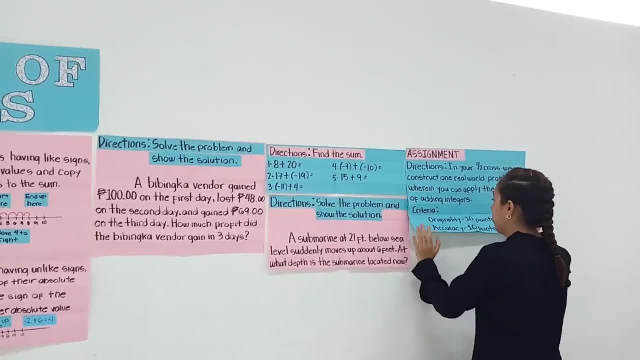 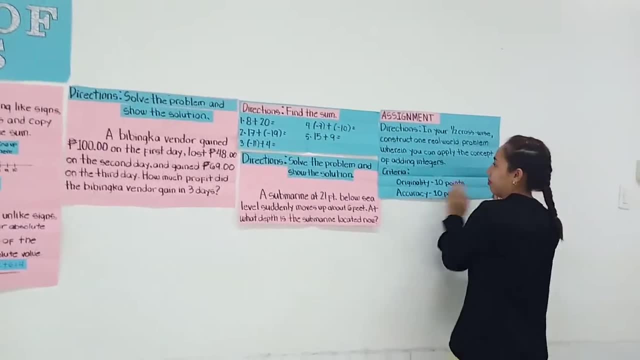 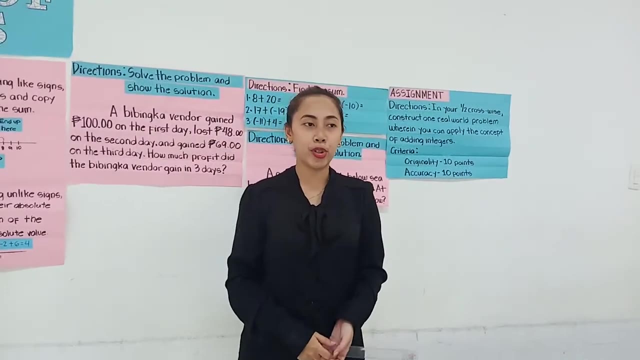